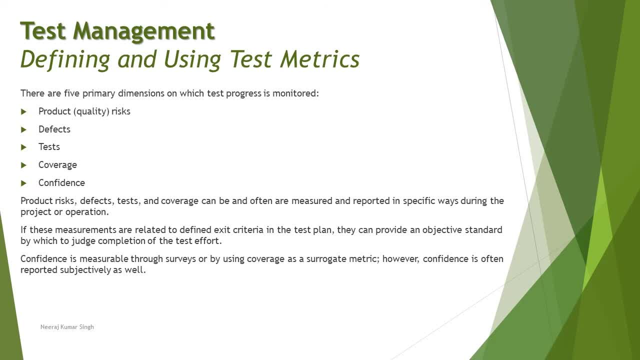 Now. so the five primary dimensions are a product risk, or can be also referred as quality risk, defects, test coverage and confidence, Of course, to understand that each one of them stand for themselves, that you know, one parameter is very important. parameter is risk, which has to be. 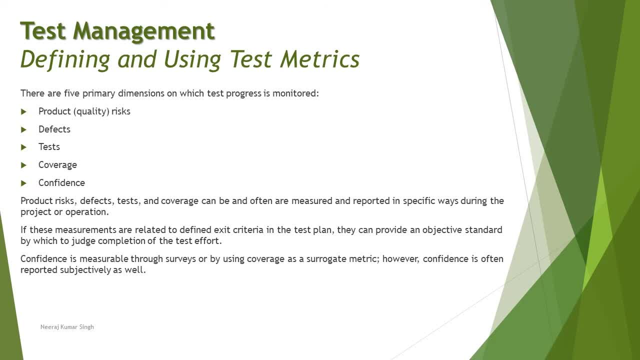 monitored from time to time in order to see whether these risks are still existing with the same severity or you have mitigated it to a certain level. Now, the first thing we are going to look at is the test level Defects. of course, each and every defect has to be captured and monitored. 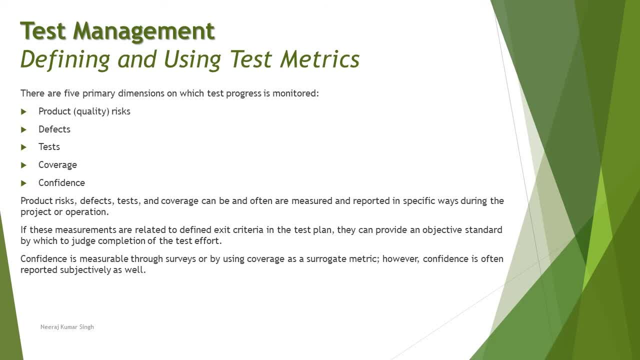 in terms of, like what number of defects you are finding, how many defects you have resolved, how many defects you have yet to resolve, and what kind of priority and severity of the defects you have, and so many things which you'll be learning in upcoming chapters as well. Test, of course, the 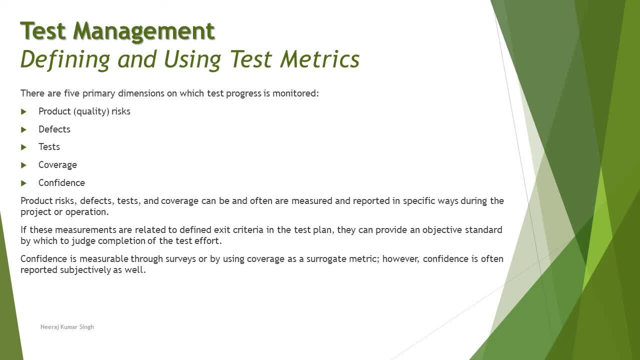 number of test cases you have created the test case, execution outcomes, the status of it and the number of test cases which were helpful in order to get good number of defects. Coverage, of course, coverage talks from the point of the overall coverage on the test or overall. 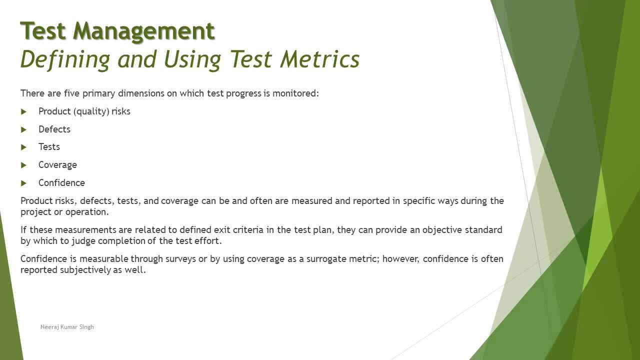 coverage on the condition statement decision. There are so many things which can be measured from the point of coverage and, of course, the confidence which basically stands for the tester's. confidence Like this is a virtual kind of thing, but of course it's yet important to be. 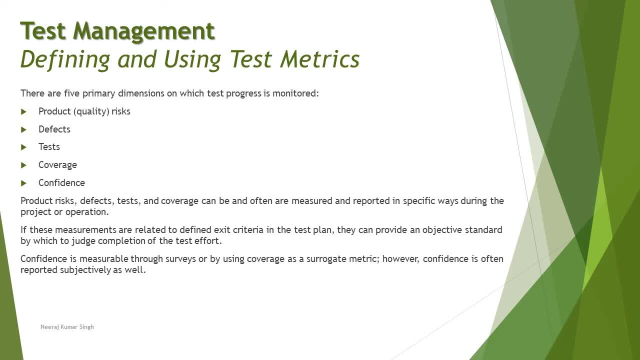 measured that? what kind of confidence does your team have on the product in order to release it? Yeah, so all the five parameters plays a vital role and covers all the requirements, Different segments in one or the other way to be measured as a part of the testing life cycle. 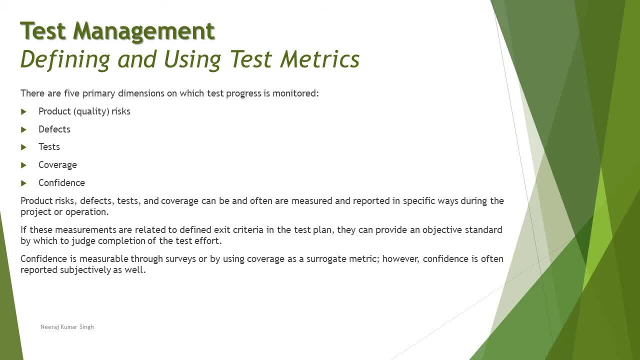 Now, these risks, these parameters, can be often measured and reported in specific ways during the project or any kind of operation which you perform in relation to that. If these measurements are related to defined exit criteria in the test plan, they can provide an objective standard by 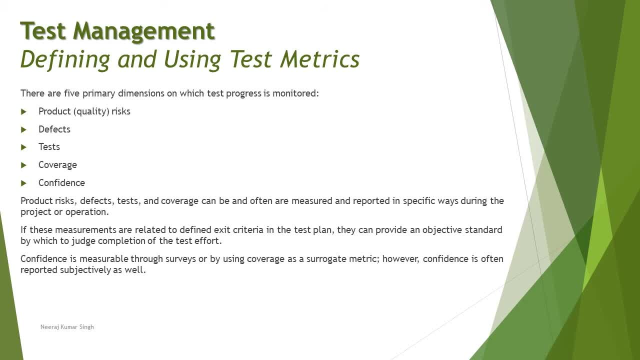 which to judge completion of the test effort. So now, if you see that these matrices are related to your exit criteria, for example, the exit criteria may have certain matrices as well, For example, number of test cases executed, number of you know the defects have been resolved. 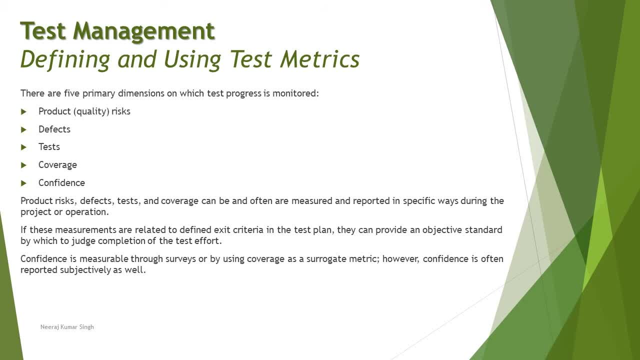 number of defects which are still open and priority one. So you know these kind of matrices can be a part of your exit criteria. So if in case they are relevant or related to your exit criteria, then of course that will also add a lot of value to be measured from time to time. 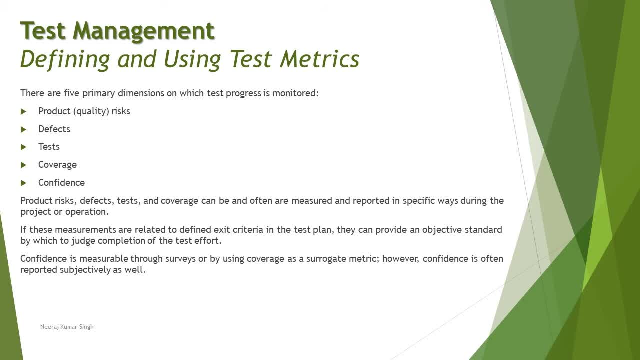 Confidence is something which is a very important part of your exit criteria, So if you have a measurable through surveys or by using coverage as a surrogate metric. however, confidence is often reported subjectively as possible, So this is basically like a kind of a debriefing session. 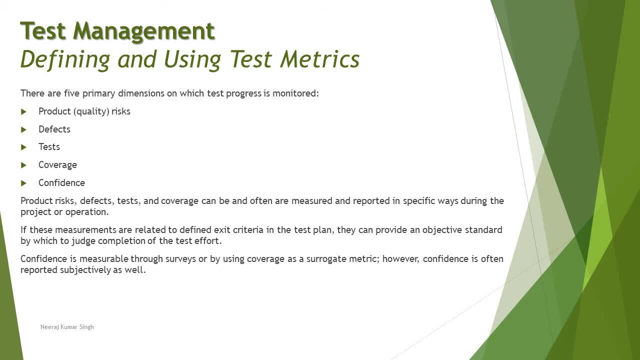 or kind of a meeting where you can generally share your experiences, share your confidence. So, to the point, you don't have any kind of calculation based driven approach. rather, you have some kind of discussion based or subjective based metrics, which is like you know. you call for a meeting and 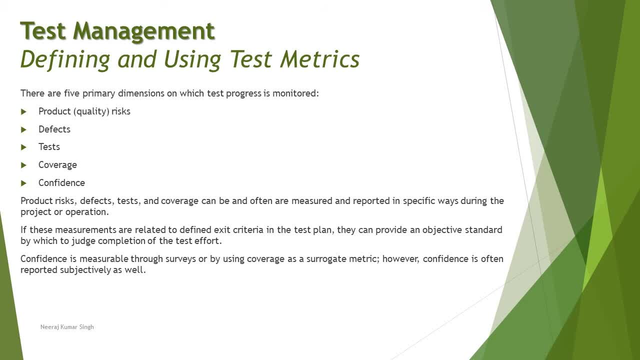 you ask your engineer to give you an answer. So this is a very important part of your exit criteria. Now, further to add, of course we are looking at some of the example matrices here and trying to understand that what kind of matrices can be used to test the product quality? So if you have a 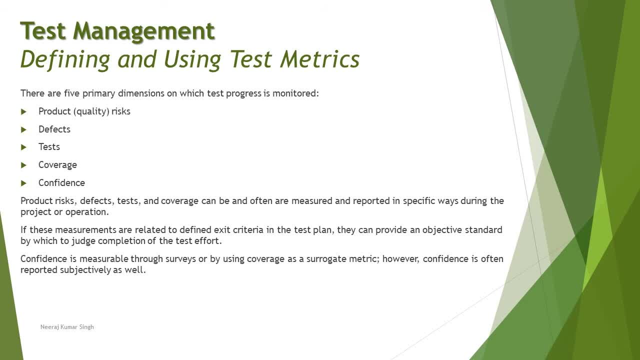 useful at what point of time? So, getting started with each parameter and trying to understand that, what kind of matrices are available for each of these primary dimensions? So starting with the very one first, that is, product risk: What kind of matrices can be used for risk associated? 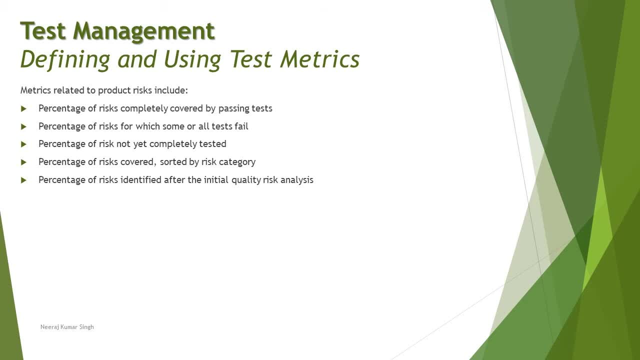 measurement of the progress, that is, percentage of risk completely covered by passing the test. percentage of risk for which some or all the tests have failed. percentage of risk not yet completely tested. percentage of risk covered sorted or risk category by risk category: percentage of risk. 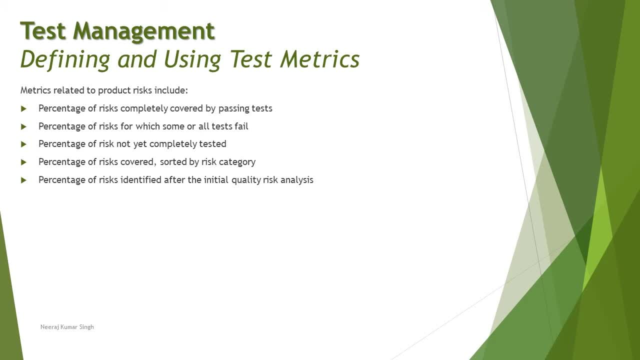 identified after the initial quality risk analysis. Now think, team. there is no explanation required because each matrix is so straightforward that it tells you what is that it will be measuring, So I will. there will be so many matrices which will be covering in today's tutorial and the next. 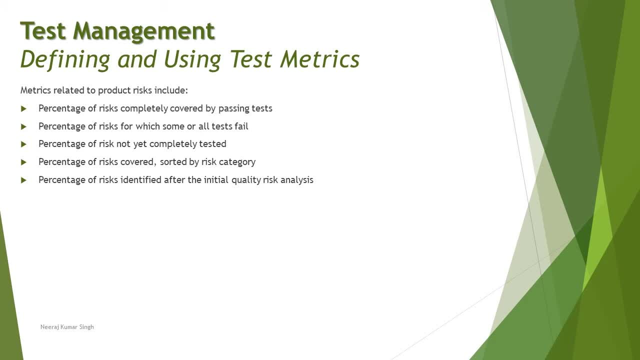 tutorial as well, So there's no point explaining each one of them. If I think that there's something which needs to be told to you about the product quality, then I will be able to explain it to you. So I will explain it in more detail, But the name here tells you that what exactly this matrix is. 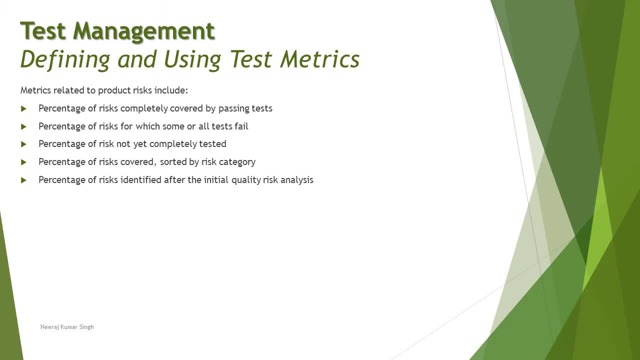 going to measure. So, being a test manager, you should be aware that. what are the possible matrices available and make use of them. If you think there's something custom which you can create, you can obviously create your own matrix, which will be adding a lot of value to your 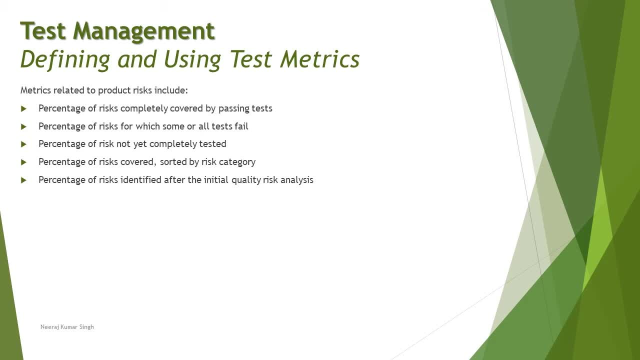 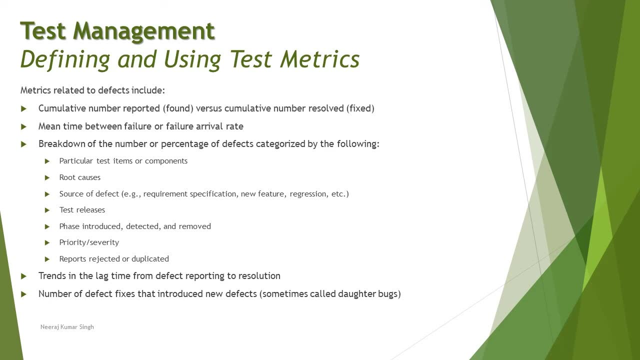 measurement. The next matrix category or the primary dimension is, of course, defects. So what kind of matrices do you need to measure? So the next matrix category or the primary dimension is: do we have, for defects, measurement on the progress? cumulative number of reported versus cumulative number of result? That's a very good comparison If you're doing that as a part of your. 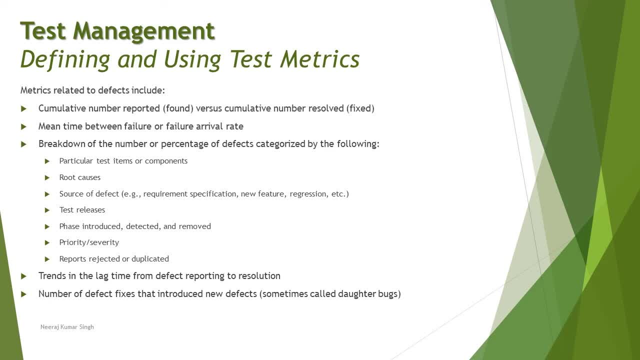 progress. you do understand that what kind of number, what number of defects you are finding and what number of results are resolving of the defects are happening, because these measurements will tell you that what is your turnaround time and how much lag do you have between the number. 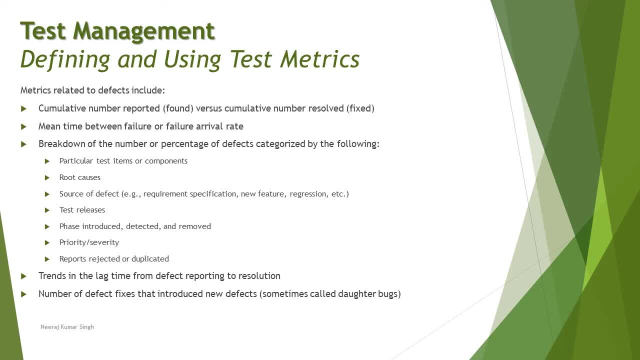 of defects being found, a number of defects being resolved, because you may have a lot of defect depth in order to resolve the defects at the end of the cycle. So keep a track of that meantime between the failure or failure arrival rate. That's another matrix which can be measured. 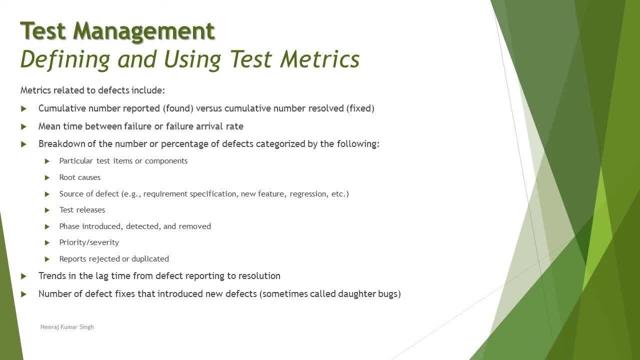 that what's the duration between two different defects being found as a part of a particular cycle. So I find a particular defect today and then I find the next defect tomorrow. That has 24 hours of meantime between failures. And the second thing could be, like you know, if every 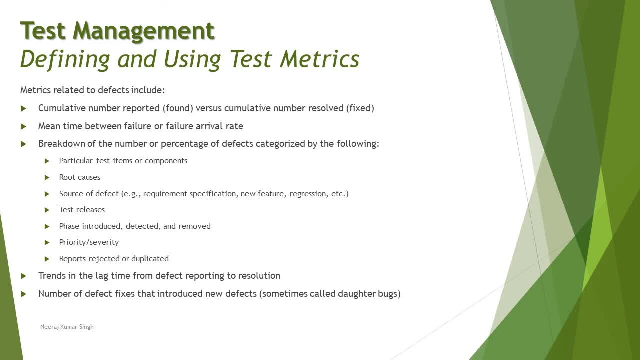 single hour you are finding a defect. So that's too huge. You know you need to worry a little bit because you need to do a lot of rework and a lot of followed following that: retesting and regression testing. breakdown of the number of percentage of defects, categorized by different. 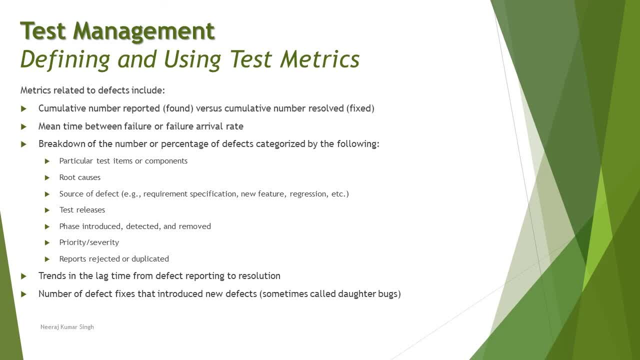 categories, Number one, particular test item or components specific to each component. what number of defects you have found? root causes, source of defect- that is like where it was initially introduced. test releases in which release phase introduced, detected and removed, priority and reports rejected or duplicated. Now you see that all these factors are one of the fields from the 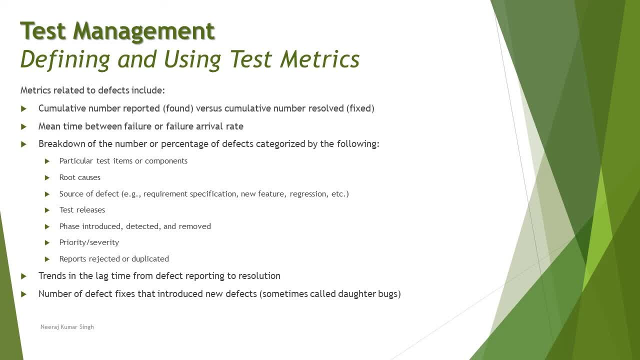 defect report and can definitely help you to measure a lot of things. Believe me on our team, the defect report alone can tell the entire organization's back end that how proficient your processes and what kind of improvement methods do you need. So defects are very, very vital in order. 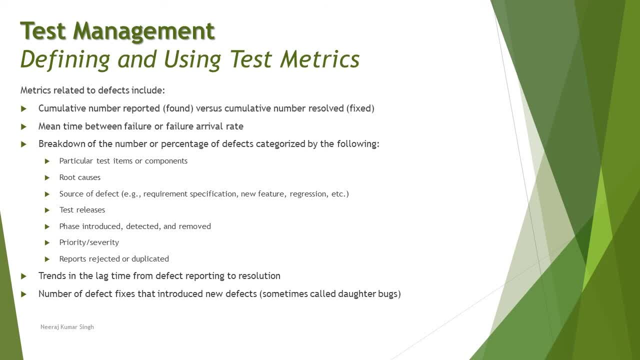 to be measured Also to add trends in the lag time from the defect reporting to the resolution, which can be done in a very, very short period of time. So if you have a defect report you can see definitely in relation to the very first matrix as well, and number of defects fixes that. 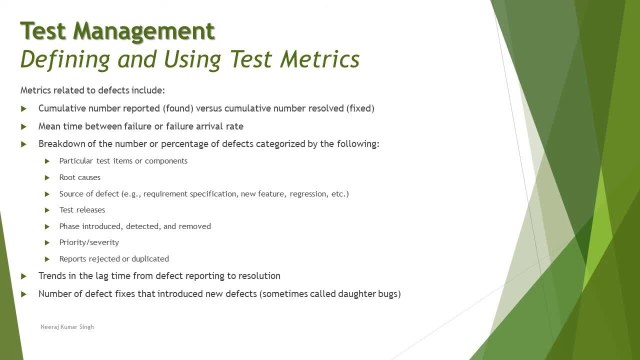 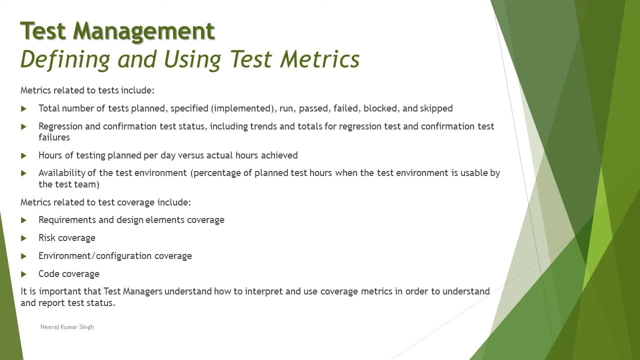 introduced new defect. that is like, of course, regression failures that due to fixing a particular defect and something else is now not working well. So these are some of the matrices which a test manager can pick from or select in order to measure the parameter defect. Similarly, if we talk about 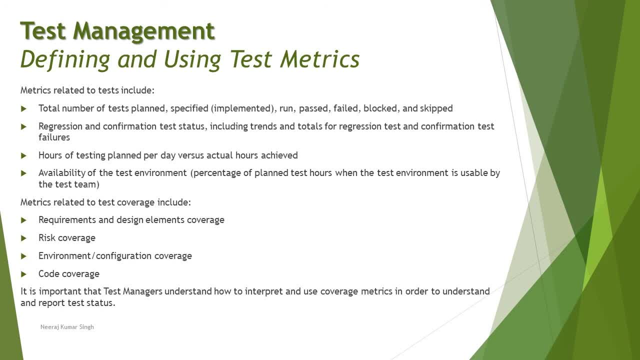 the other option, that is, the test. of course, for the test as well, you do have a lot of matrices. so total number of tests planned, specified, that is, implemented, run, passed, failed, blocked or skipped. So this is completely specific to test cases which you have written or the test script which you have. 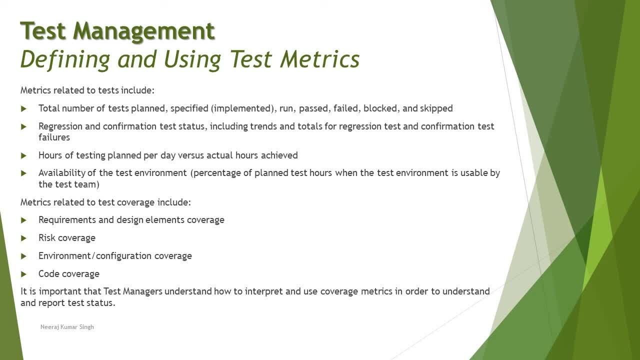 executed and you do manage the status of that. So what kind of status do you have on these matrices- Regression and confirmation test status, including the trends and totals for regression test and confirmation test failures? So both the things: number of confirmation test failures, total number of test failures, total number of test failures. 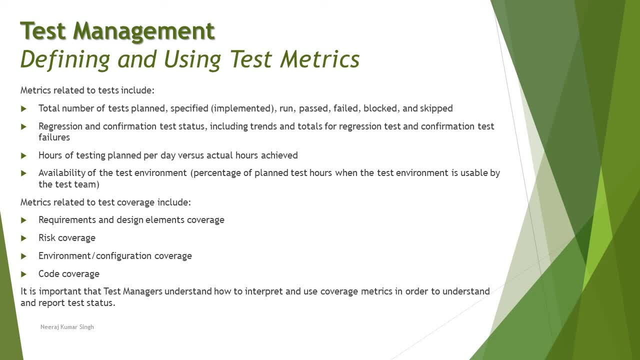 number of confirmation and regression test execution follow that. what kind of status does that have? whether, how many of them passed? how many of them failed? if they failed, what's the number of that? because how many you know? defect resolutions are not effective, So we can talk about it probably. 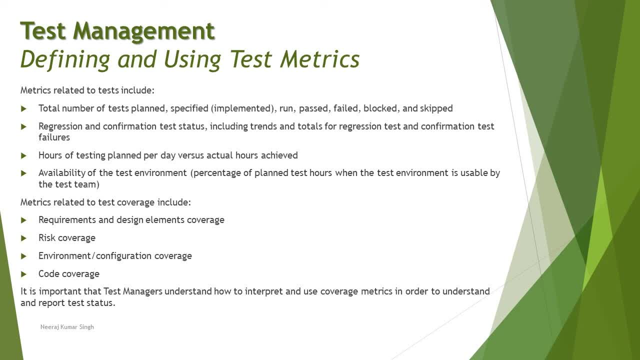 like on, out of 50 confirmation tests, you know 50 out of 50, 30 of them are failing. That means you know they're. fixing of the resolution or fixing of the defects are not so effective, So we need to talk to the developers in order to tell them. 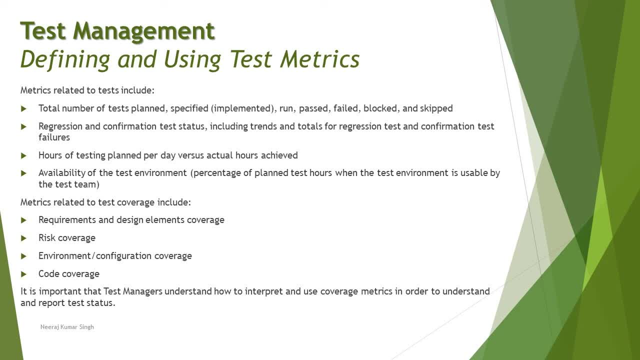 that you do try to resolve the issues, but things are not working on the other side And we are actually investing a lot of time and waiting for your resolutions to happen so that we can proceed further. So sometimes your defects can be probably a blocker as well, And you don't want to, you know. 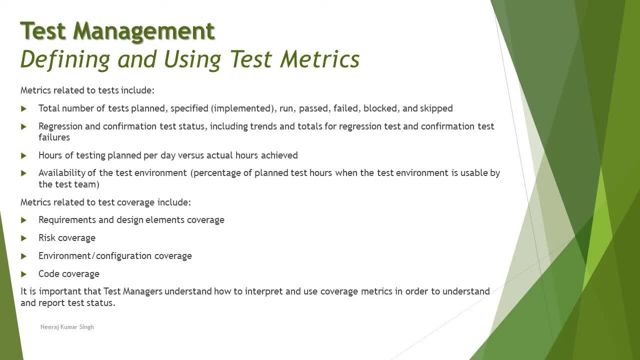 stay up for a long time on a particular module. You do have to test a lot of other things: Hours of testing planned per day versus actual hours achieved. Of course, comparison of the effort, what you're putting, availability of the test environment. 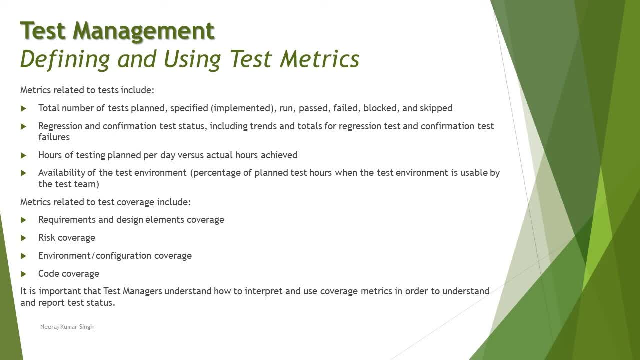 as the percentage of planned test hours when the test environment is usable by the testing. So, number of time or number of hours, what you allocate in order to do any particular activity here, in this case, it is the test environment, preparation and availability. So all these things. 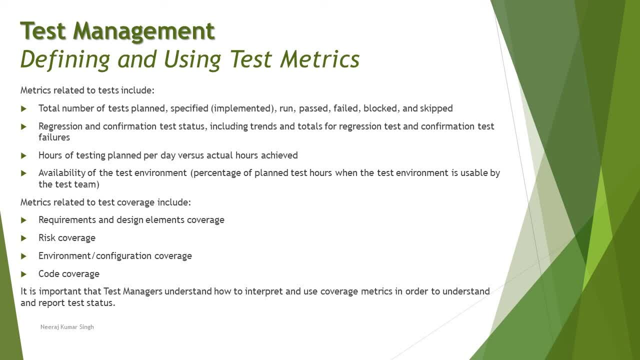 can also be measured, So this is just not limited. Okay, These are just some of the typical examples of matrices. There are many of those which you can definitely find specific to each one of them. Well, also to add a matrices related. 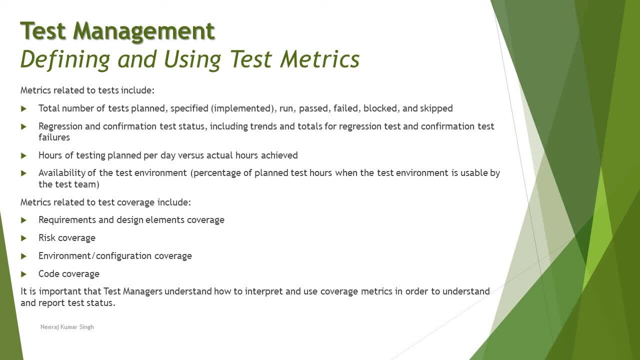 to the test coverage. Now, matrices related to the test coverage measurement includes requirement and design coverage, risk coverage, environment and configuration coverage or code coverage. So these coverages basically stand for that. For example, if I have a requirement, then what number of test cases I've written, whether these test cases which I have written. 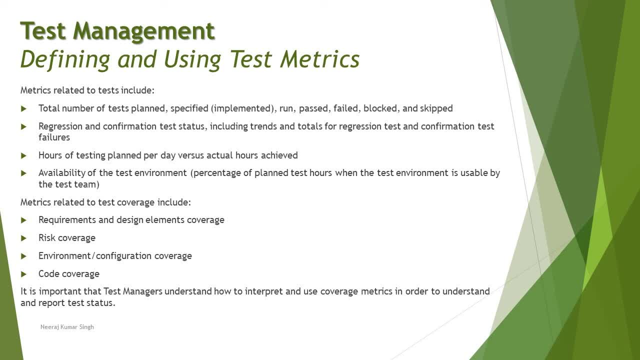 is covering all the aspects of the requirement or not. Similarly, if you talk about the design, you talk about the risk, you talk about the code. So what number of test cases you've written, and whether these test cases are enough to have a hundred percent coverage, or what percentage? 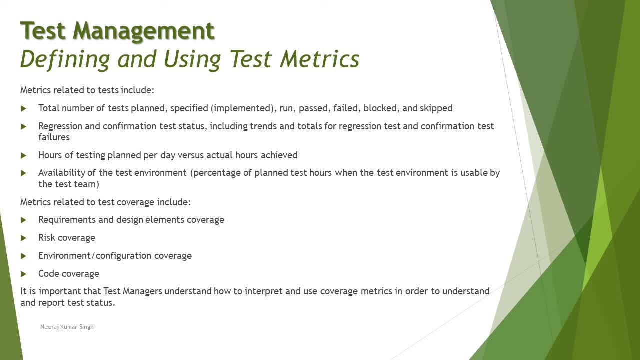 of coverage you have you achieved by writing these test cases. So you know all these matrices will definitely add a lot of value from time to time to determine that how much coverage you have achieved and what more you can do in order to add more value. It is very important for that, the test 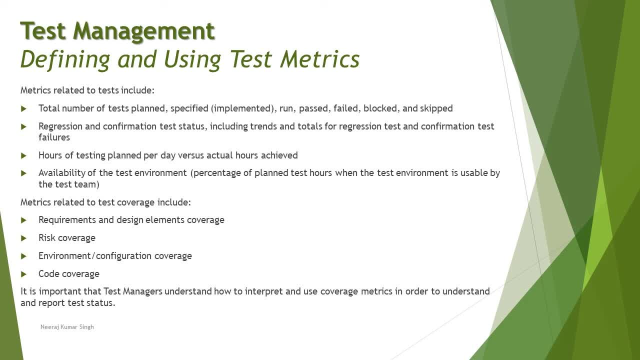 manager understands how to interpret and use coverage matrices in order to understand and report the test data. So now that's a very critical responsibility of the test manager from time to time to keep an eye on making use of several matrices and decide that what kind of matrices will be best applicable, and also put it in such 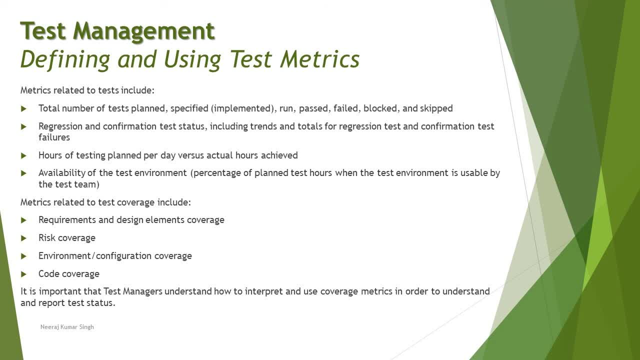 a way that it is measurable and it is representative to different stakeholders. so, if you remember from the previous tutorial, we did talk about it and that's what we need to take care of, and at any point of time, the test manager can determine further measurements of certain specific matrices.